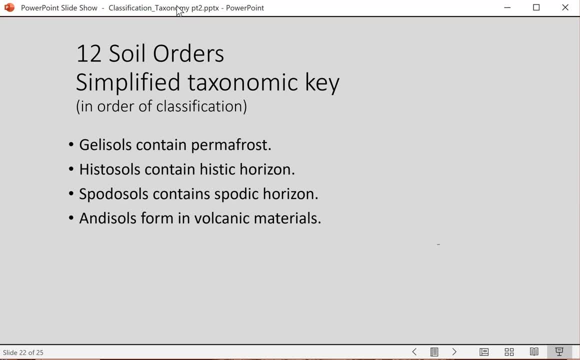 Andesols form in volcanic materials. You have these in the Pacific Rim. You have some in the Pacific places where there have been active volcanoes in the past and a climate that's sufficient for a soil to form. Then oxosols are extremely weathered soils. They have an 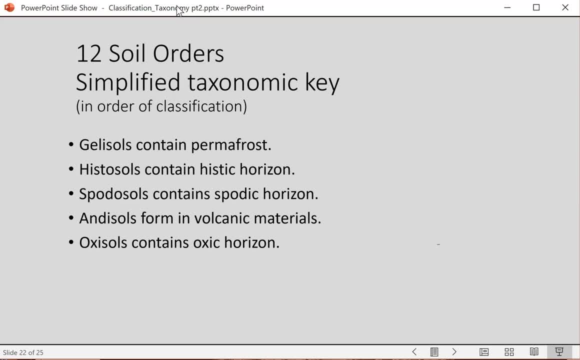 oxic horizon. You find most of these in the tropics. In the US, Hawaii is an example where you find many oxosols. Vertisols contain slickensides. These are soils with a great deal of shrink swells. You can find a lot of these in the Pacific Rim. You can find a lot of these in the. 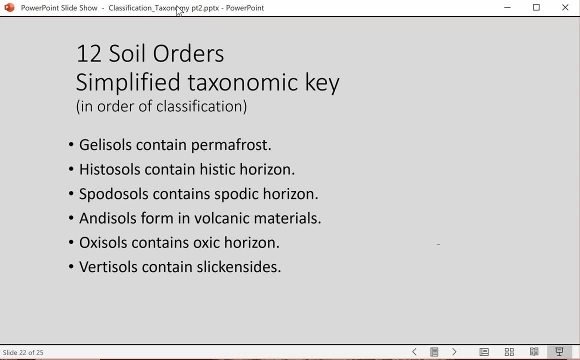 swell clays, and so there's a lot of movement that can limit soil development, and these slickensides are unique features that you can observe, associated with the soil structure. So if you find vertisols, it's going to be a vertisol. Slickensides, it's a vertisol. 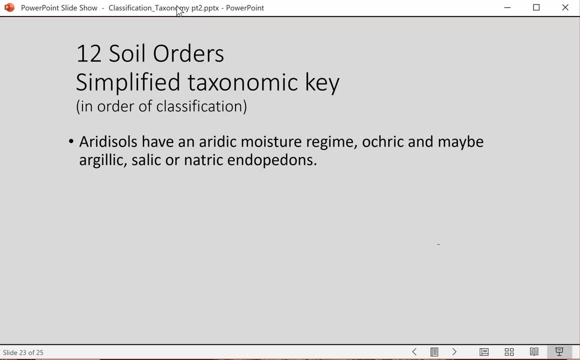 Going on, and this one is one that gets a lot of debate because it's the only one that has been classified according to its climate, as opposed to the characteristics and features of the soil. So does it have an aridic moisture regime? Is it dry most of the year in the 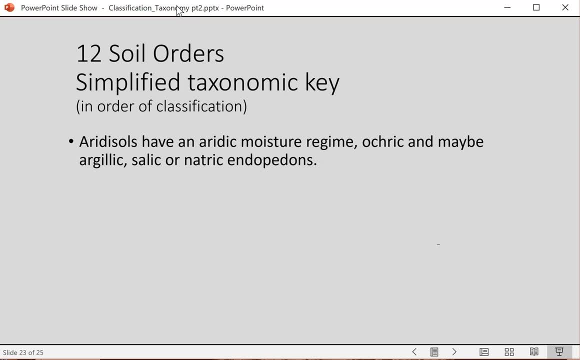 soil profile. It may have an ochric horizon at surface generally and then in the subsurface it may have a series of things. It could have argillic or salic or natric or calcic or petrocalcic, all sorts of 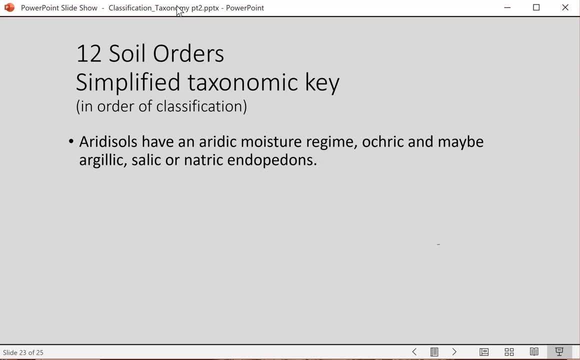 things that could be gypsic That you can find there, and so it's probably the broadest category in terms of soils that have some degree of development, because it's based on the climate, and the challenge with that is the climate may not have always been as it is now. 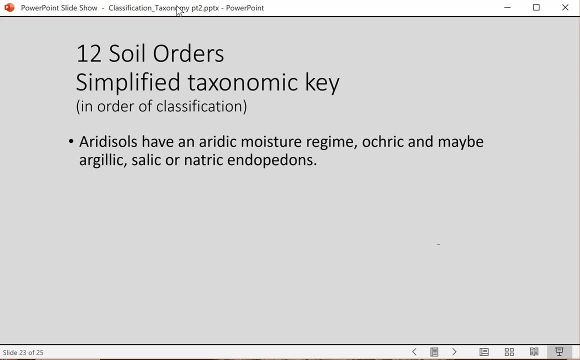 and so a lot of that soil development may have happened in the past in previous climates in that region. Ultasols. then they have an ochric surface horizon, low organic matter and argillic horizons in the subsurface. Those are the accumulations of clay. 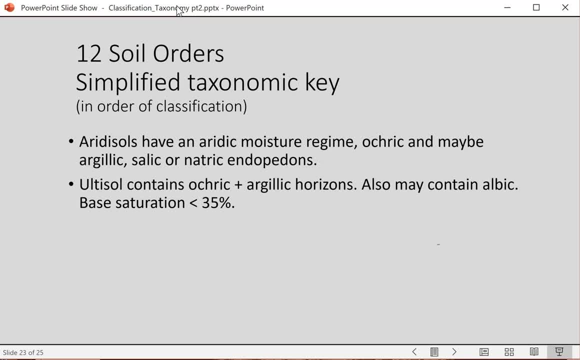 They can also have an E or albic horizon zone of loss and their base saturation is less than 35% in the B horizon. This means that they tend to be more acidic and less fertile. You find a lot of these in the bands around the tropics north and south of them. 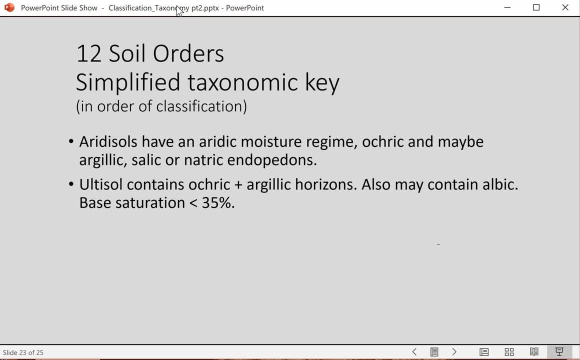 so in the subtropical regions In the US you usually have to get south into Arkansas before you can find these parts of Oklahoma, so areas with warmer temperatures and higher rainfall that result in greater degree of weathering in the soil, So greater degree of transformation and 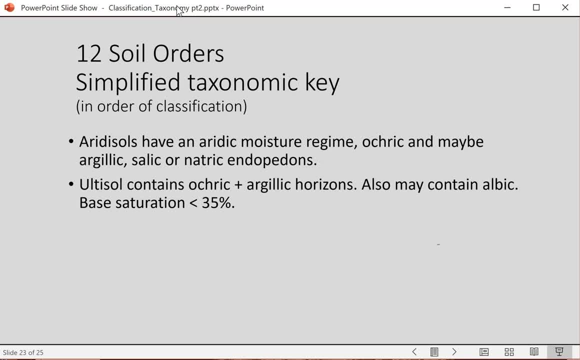 losses of the calcium and magnesium things that hold the pH up. Then a mollisol contains a mollic horizon, the epipedon key. a mollic horizon is one that has soil structure. It has the dark colors, value in chroma of 3 or less. It has an organic carbon content. 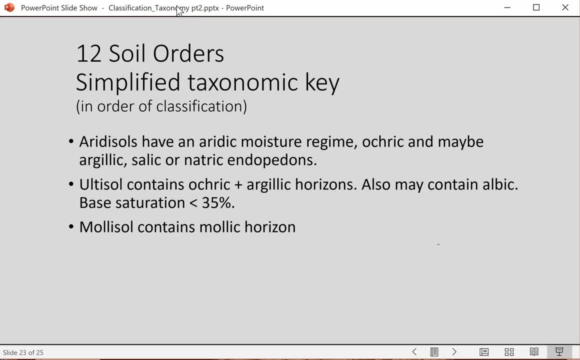 greater than 0.6% or 1% organic matter And it has a base saturation percentage greater than 50%. Typically, these are associated with our grasslands, And so if all those features meet, it's a mineral horizon. then you have a. 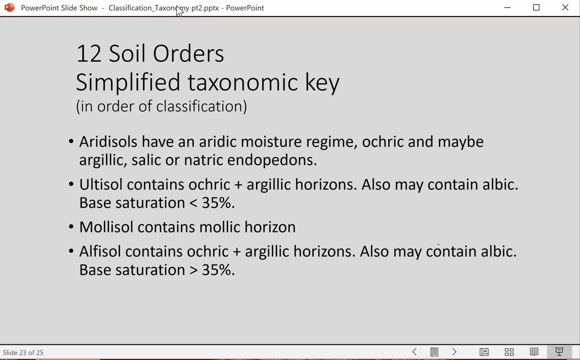 mollic horizon and a mollisol. Then we come to the next one. Mollisols also often have argillic horizons, but the mollic part horizon takes precedence in the classification. It controls more of the soil properties. Then an althisol has an. 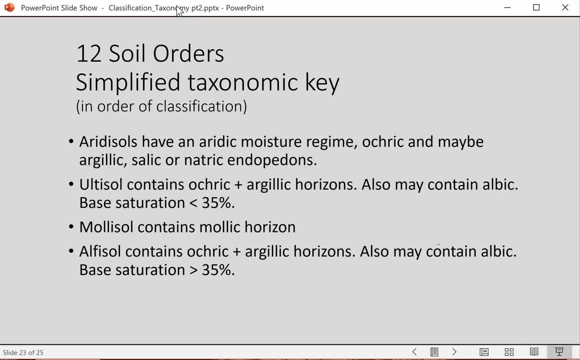 ochric horizon plus an argillic horizon. Those are mandatory things. Sometimes an althisol may have an umbric horizon. They also may have an albic horizon Contrasting those to the ultasol. they have more basic cations. 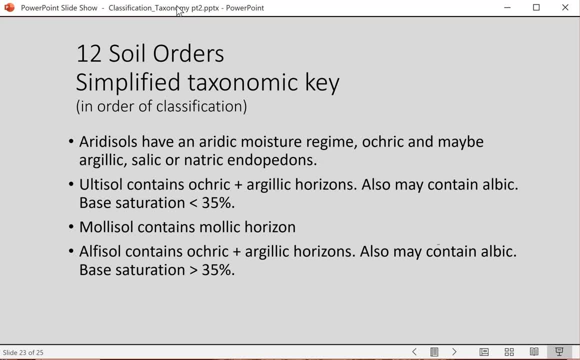 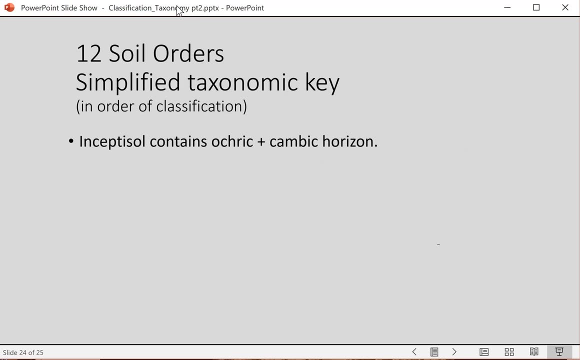 calcium magnesium and such that hold the pH up a little bit higher and make these a little more fertile. You find these generally a little further north than you find the ultasols, where weathering conditions have been a little less severe. We continue, We're down to our last two. An inceptosol has a weak